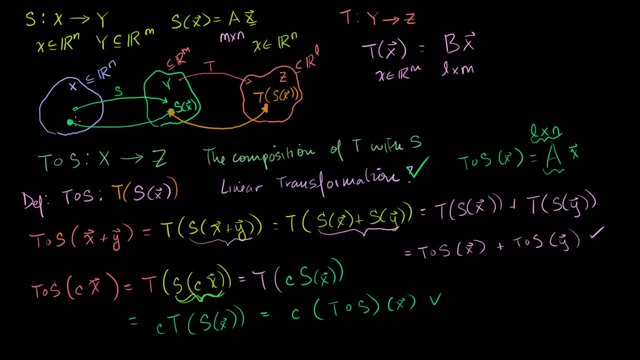 And what that is is: first you apply S to some vector in X to get some vector in Y, And that's your vector right there, And then you apply T to that to get to Z, And so we defined it that way. And our next question was: was that a linear transformation? 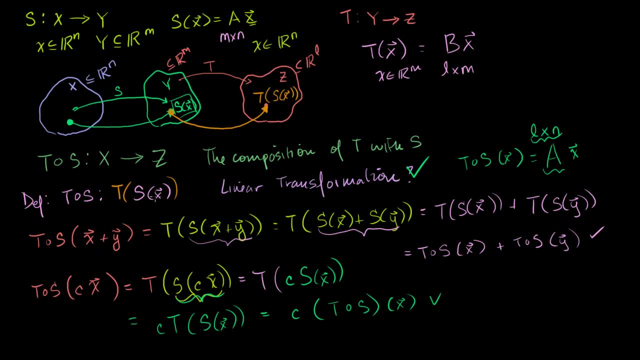 We showed that it was. It met the two requirements for them And because it is a linear transformation, I left off in the last video saying that it should be able to be represented by some matrix vector product, where this will have to be an L by N matrix. 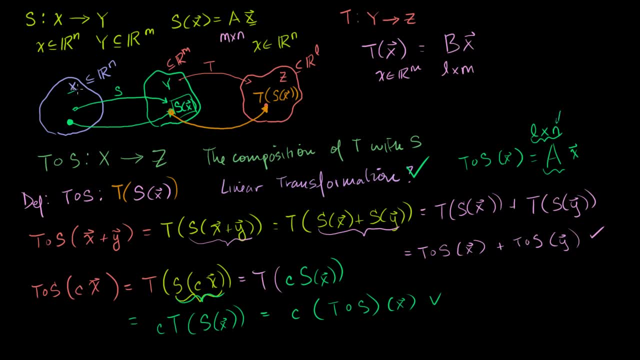 Because it's a mapping from an N-dimensional space, which was X- it was a subset of Rn- to an L-dimensional space, Because Z is a subset of RL. Now, in this video, let's try to actually construct this matrix. 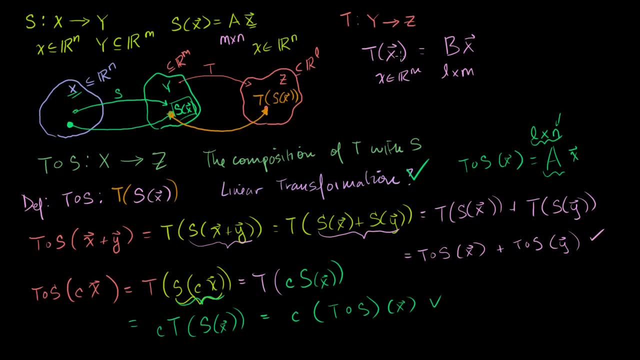 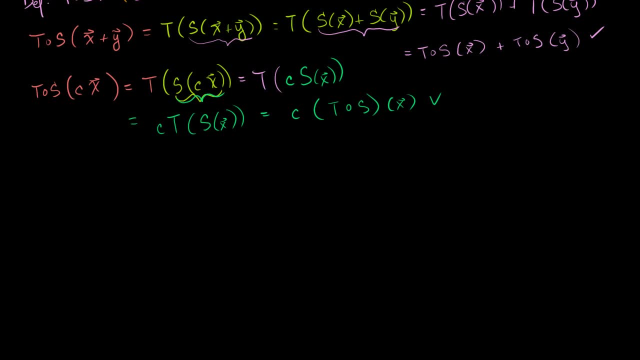 So at the beginning of the last video I told you that T of X could be written as some matrix product B times X. Let me write that, Let me rewrite it down here. So I told you that the linear transformation T applied to some vector X could be written as the matrix vector product B. 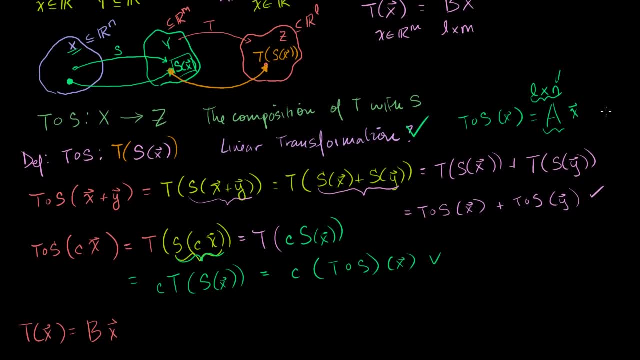 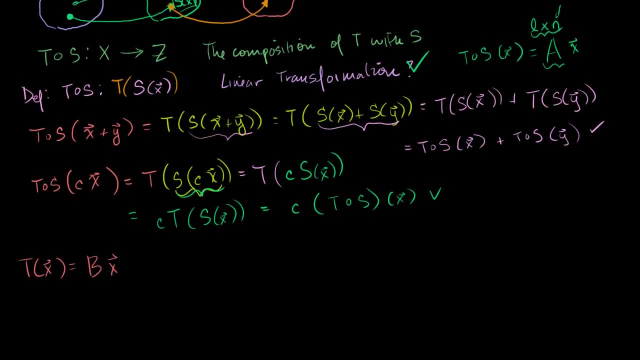 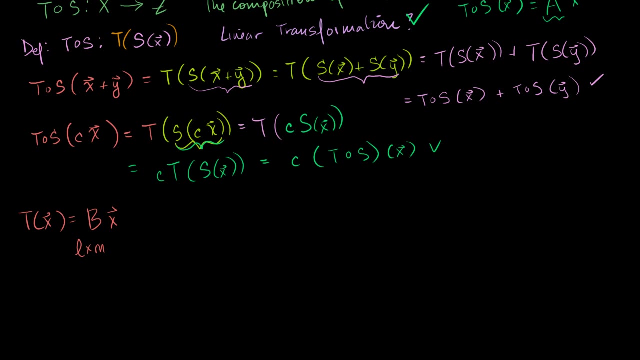 times the vector X And since it was a mapping from a M-dimensional space to an L-dimensional space, we know that this is going to be an L by M matrix. Now, similarly, I told you that the transformation S can also be written as a matrix vector product, where we could. 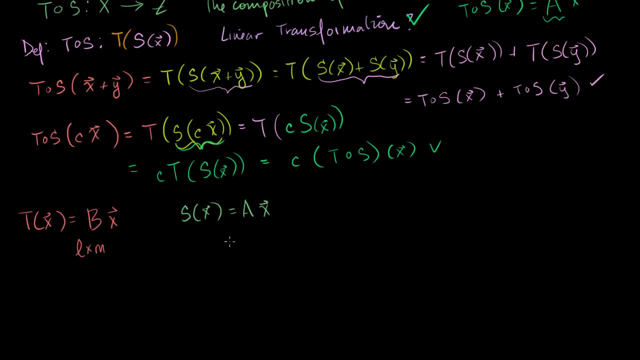 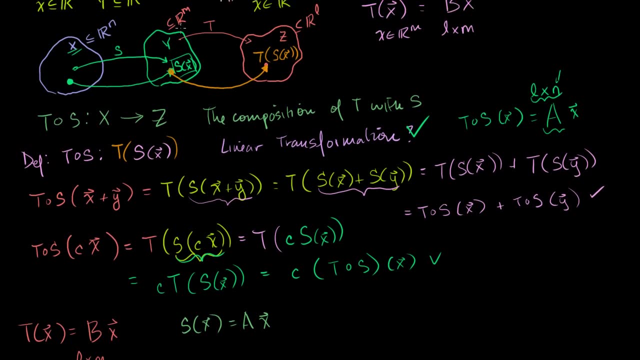 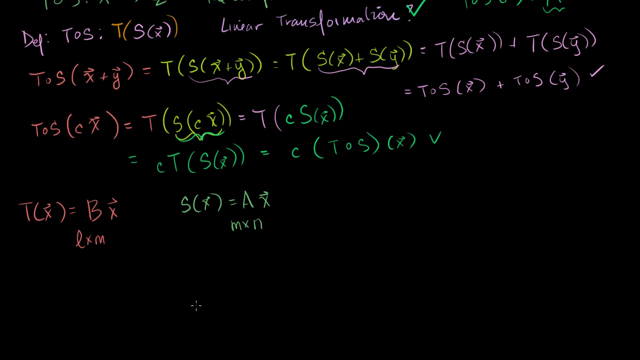 say, maybe A is its matrix representation times the vector X, And since this is a mapping from a- remember S was a mapping from a N-dimensional space to an M-dimensional space- this will be an M by N matrix. Now, by definition, we're going to be able to do this. 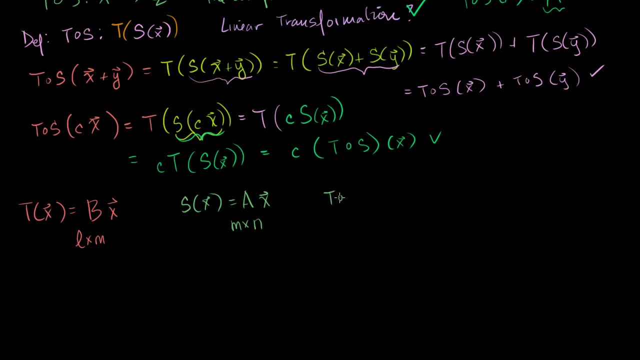 By definition? what was the composition of T of S, T with S? What is this By definition? we said that this is equal to. you first apply the linear transformation S to X and I'll arbitrarily switch colors. So you first apply the transformation S to X and. 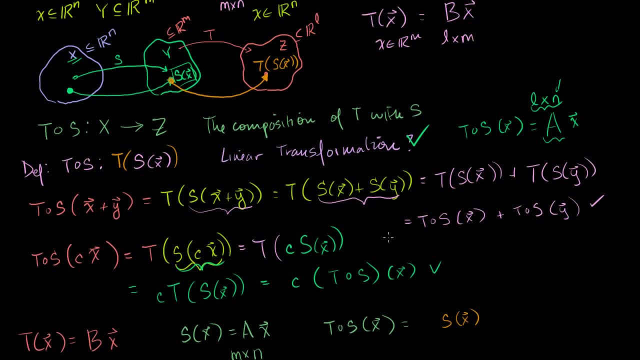 that essentially gets you a vector right there. This is just a vector in Rm, or it's really a vector in Y, which is a subset of Rm, And then you apply the transformation T to that vector to get you into Z. 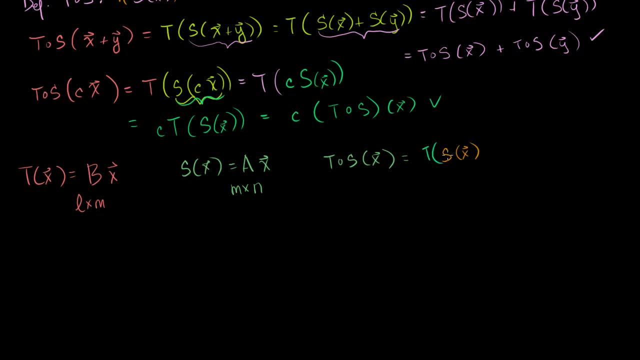 So then you apply T to that, You apply T to that. Well, given this, we can use our matrix representations to replace this kind of transformation representation, although they're really the same thing. What is a transformation of S applied to X? 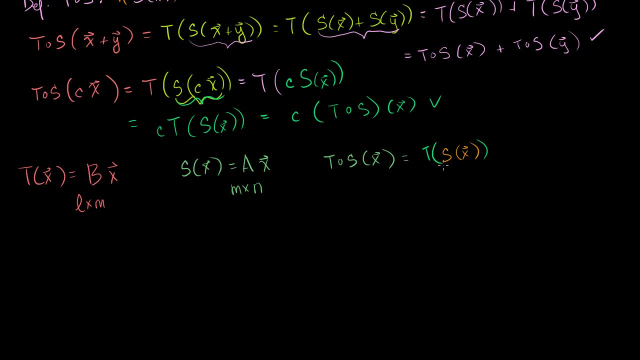 Well, it's just this right. here is just A times X. That is just A times X. Where this is an M by X, This is an M by N matrix, So we could say that this is equal to the transformation applied to A times X. 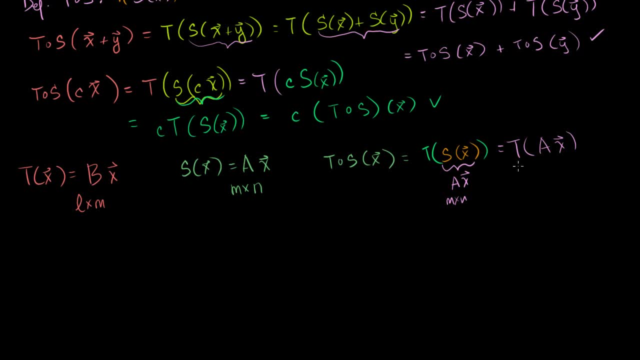 Now, what is the transformation of? what is the T transformation applied to any vector X? Well, that's the matrix B times your vector X. So this thing right here is going to be equal to B times whatever I put in there. So the matrix B times the matrix A times the matrix X. 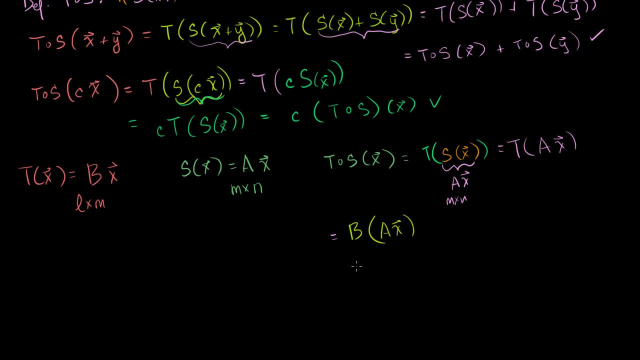 So that's the matrix B times your vector X, So that's A times the vector X. right there, This is what our composition transformation is. The composition of T with S applied to the vector X, which takes us from the set X all the way to the set Z, is this if 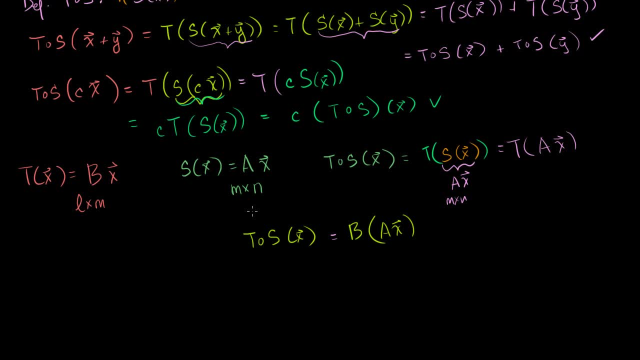 we use the matrix forms of the two transformations. Now we know that we can. you know, at the end of last video I said I wanted to find just some matrix that, if I were to, you know, multiply it times this vector. that is equivalent. 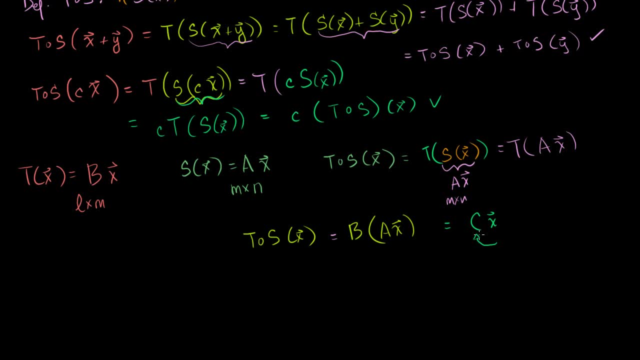 to this transformation, And I know that I can find this matrix. I know that this exists because this is a linear transformation. So how can we do that? Well, we just do what we've always done in the past: We find, we start with the identity matrix and we apply. 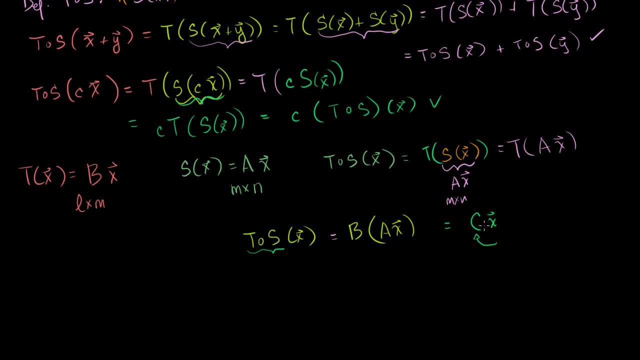 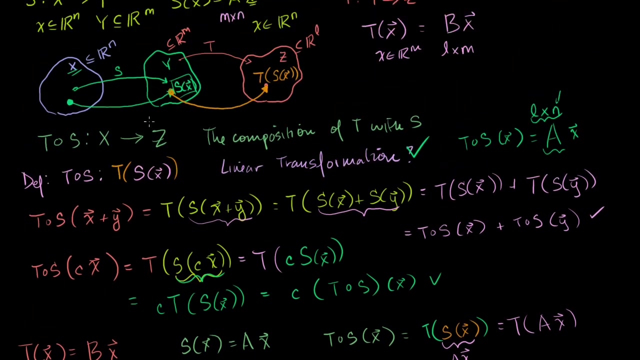 the transformation to every column of the identity matrix, And then you end up with your matrix, representation of the transformation itself. So, first of all, how big is the identity matrix going to be? Well, these guys that we're inputting into our transformation, they are subsets of X or they're members of X. 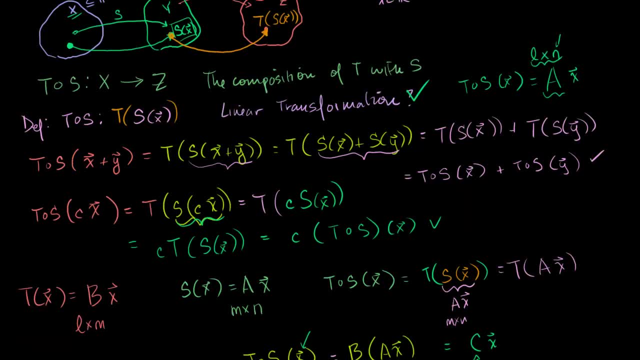 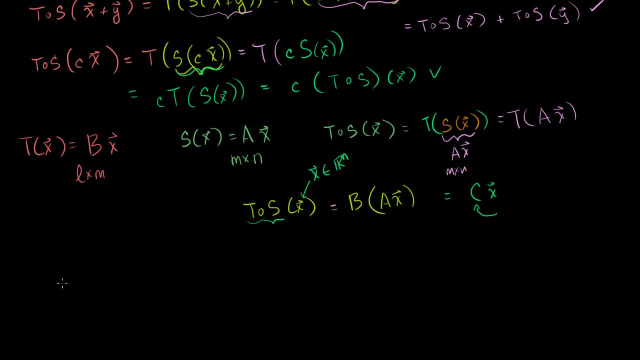 which is an n-dimensional space, the subset of Rn. So these, let me write this: X is a member of Rn. So all we do to figure out C is we apply. so we start off with the identity matrix. So let's see, we start with the identity matrix, the 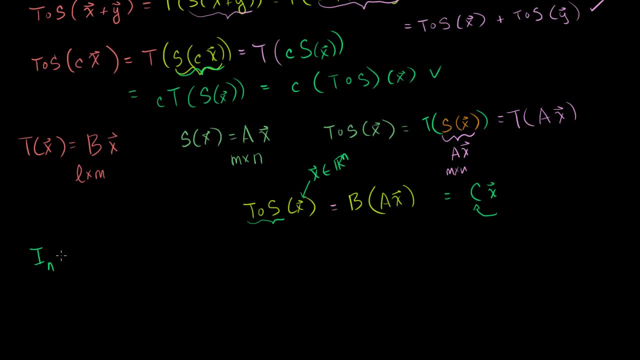 n-dimensional identity matrix, because we're starting, our domain is Rn And of course we know what that looks like. Let me draw a little straighter. We have 1, 0,- all the way down- It's going to be an n-by-n matrix- and then 0, 1,- all the. 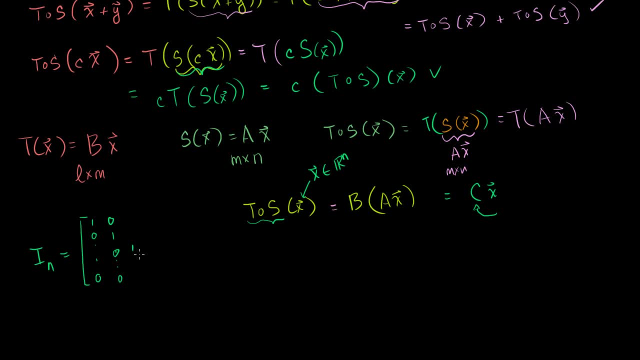 way down 0's. these are 0's right here, and then you have 1's. go all the way down the columns and everything else is 0. We've seen this multiple times. That's what your identity matrix looks like: just 1's. 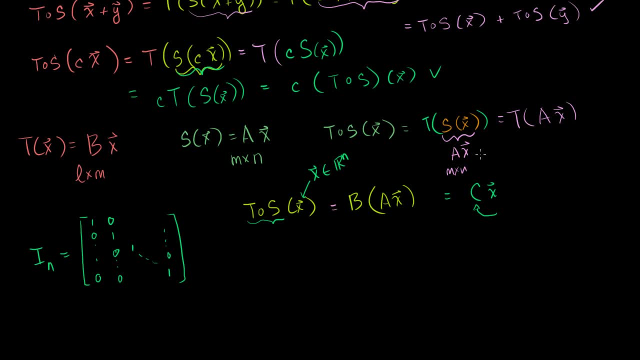 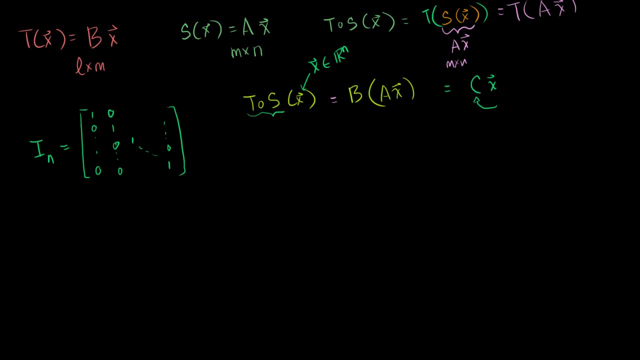 down the column from the top left to the bottom right. Now to figure out C. To figure out C, the matrix representation of our transformation, all we do is we apply the transformation to each of these columns So we can write that our matrix C is equal to it's. 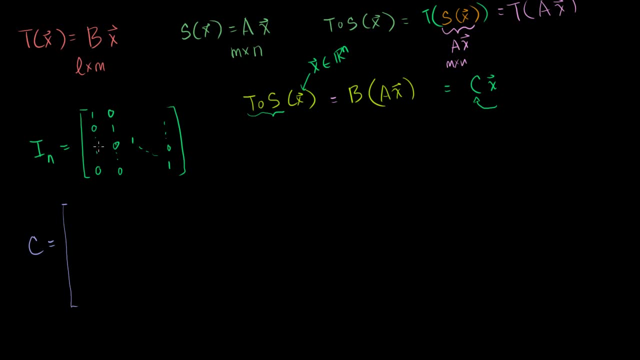 going to take some space here. the transformation applied to this first column. But what is the transformation? It is the matrix B times the matrix A times. whatever you're taking the transformation of, In this case we're taking the transformation of that. 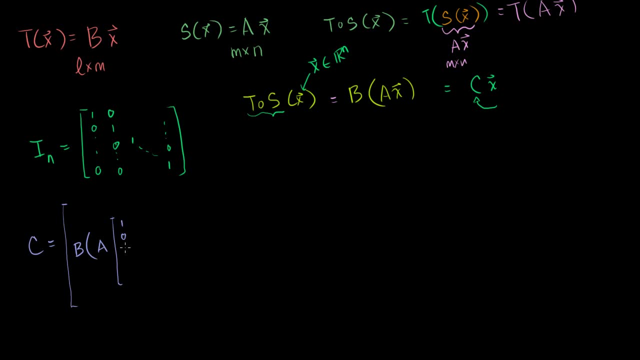 So we're taking the transformation of 1, 0, 0, all the way down. There's a bunch of 0's. 1 followed by a bunch of 0's. That's going to be our first column of C. 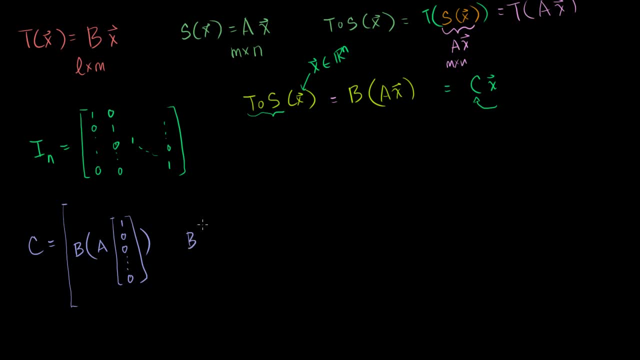 Our second column of C is going to be B times A times the second column of our identity matrix And of course you remember, these are each the standard basis vectors for Rn. So this is E1,, this is vector E2.. 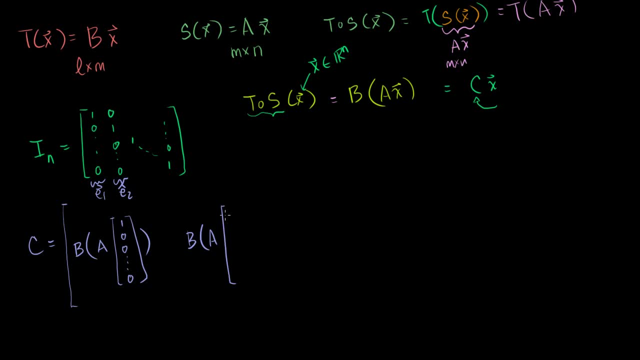 I could actually put a hat there, because they're unit vectors. You know that already, So this is going to be times E2, which is 0,, 1,, 0,, all the way down a bunch of 0's. 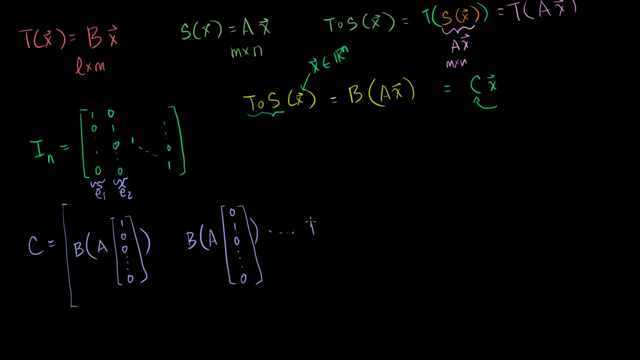 And then we're going to keep doing that until we get to the last column, which is B times A times a bunch of 0's all the way down and you get a 1.. The nth term is just a 1, right there. 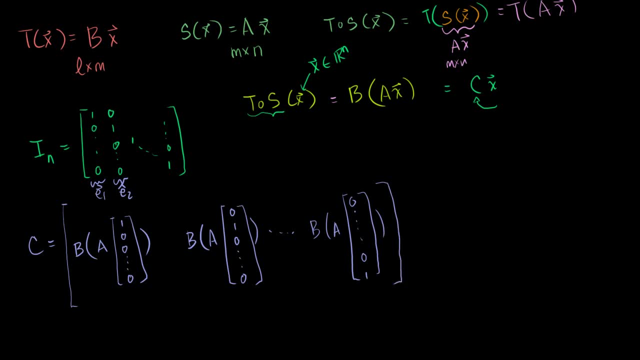 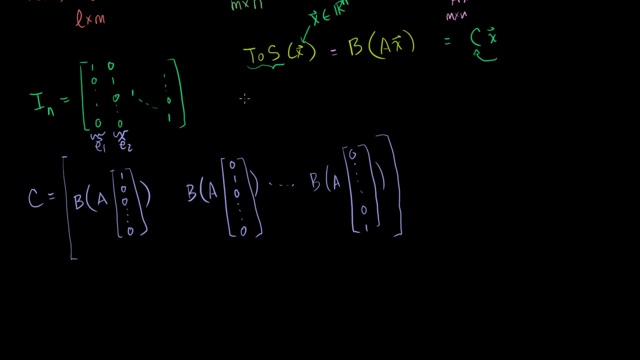 Now what is this going to be equal to? It looks fairly complicated right now, but all you have to do is Make the realization- and we've seen this multiple times- that look, if we write our vector A or we write our 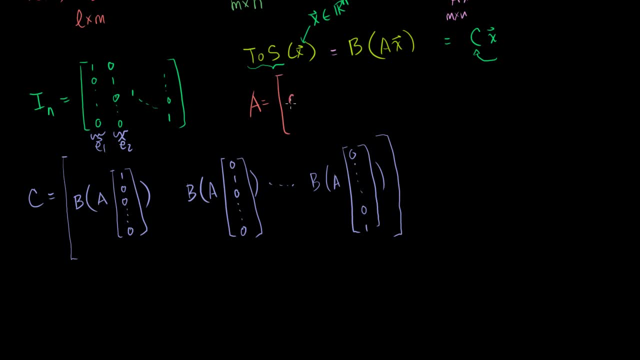 matrix A as just a bunch of column vectors. so this is the column vector A1, A2, all the way to An right. We already learned that this was an n by m matrix. Then what is the vector A times, for example, 1,. well, 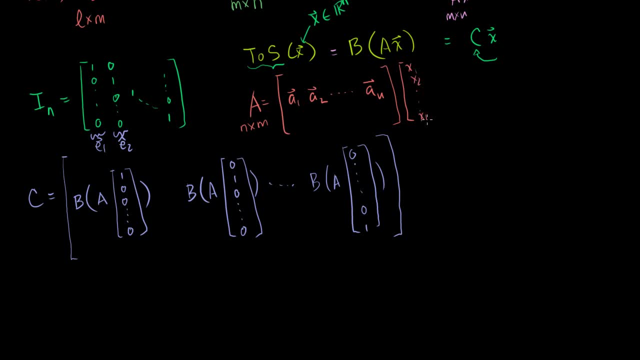 actually let me write it this way- Times x1. x2, all the way down to xn. We've seen this multiple times. This is equivalent to x1 times A1, plus x2 times A2,, all the way to plus xn times An. 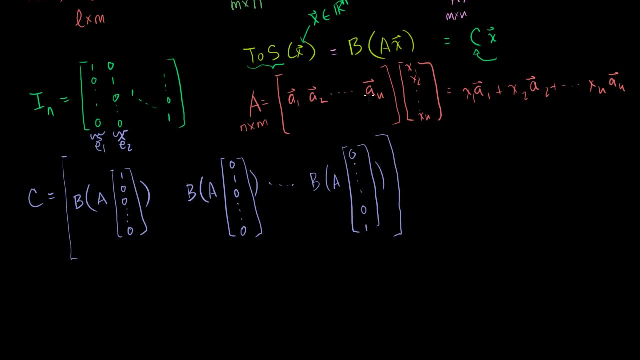 We've seen this multiple times. It's a linear combination of these column vectors where the weighting factors are the terms in our vector that we're taking the product of. So, given that, What is this guy going to reduce to? This is going to be A1 times this first entry, right here. 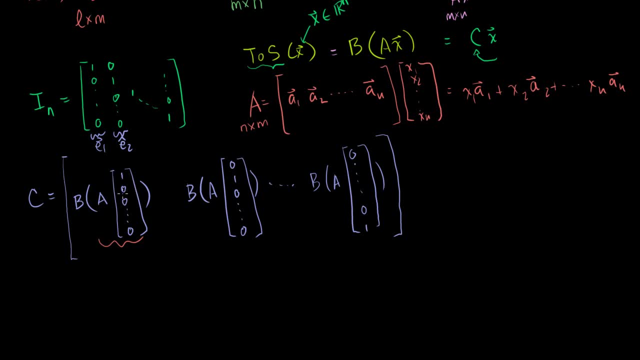 times x1, plus A2 times the second entry, plus A3 times the third entry, but all these other entries are 0.. The x2's all the way to the xn are 0. So you're only going to end up with 1 times the first column. 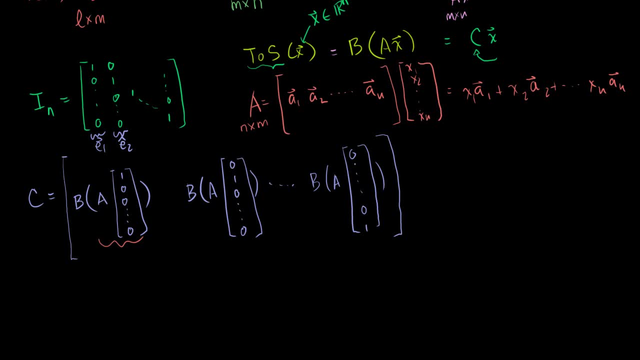 here in A, So this will reduce to. let me write this: So C will be equal to the first column is going to be B times now A times this E1 vector. I guess we could call it the standard basis vector, right there. 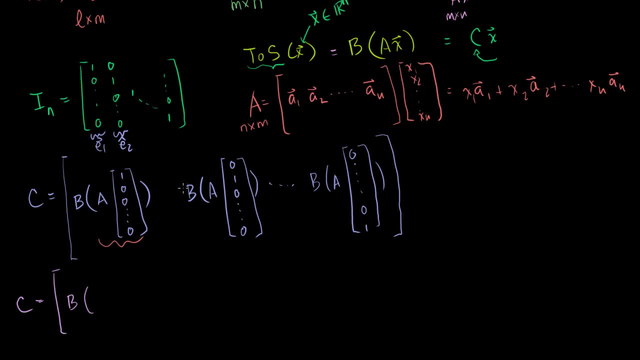 We already said, it's just going to be 1 times the first column in A, plus 0 times the second column in A, plus 0 times the third column, and so on and so forth. So it's just 1 times the first column in A. 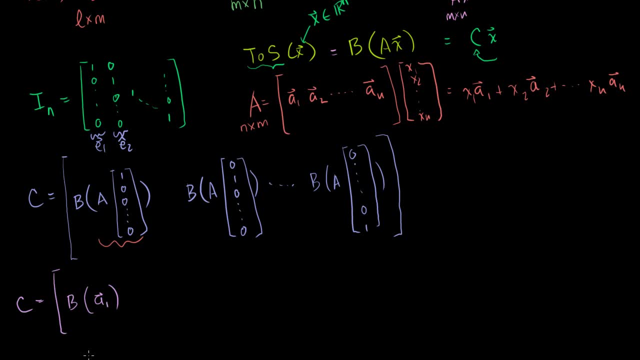 So it's just A1.. That simple. Now, what is this one going to be equal to? Well, it's going to be 0 times the first column in A, plus 1 times the second column in A, column in A plus 0 times the third column in A and the. 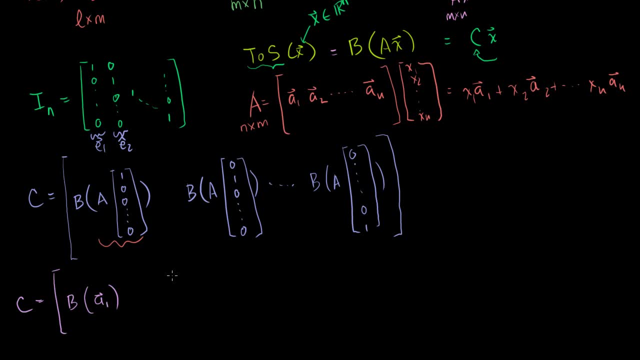 rest are going to be 0. So it's just going to be 1 times the second column in A. So this second column in our transformation matrix is just going to be B times A2.. And I think you get the idea here. 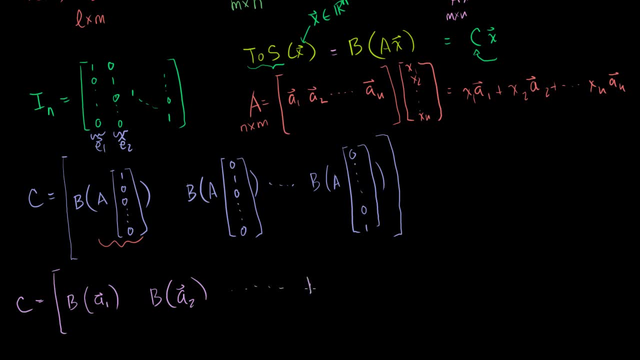 Each of these. the next one's going to be B times A3, and all the way until you get B times An. All the way until you get B times An, And so that's how you would solve for your transformation matrix. Remember what we were trying to do. 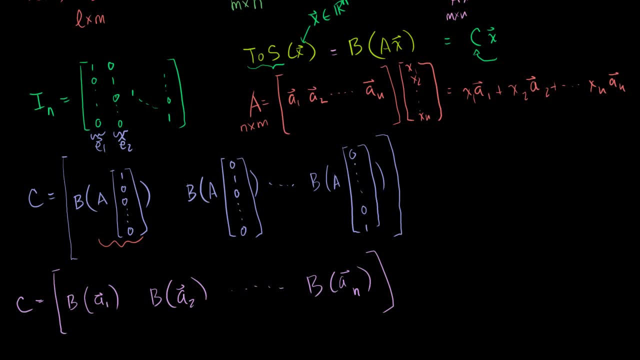 We were trying to find some. let me write down, kind of summarize everything that we've done so far. We had a mapping S that was a mapping from X to Y, But X was a subset of Rn, Y was a subset of Rm. 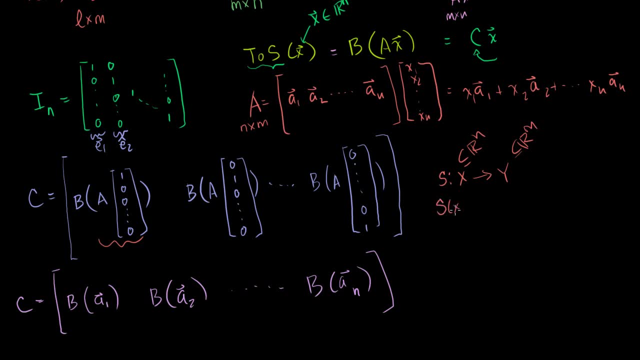 And so we said that this transformation, this linear transformation, could be represented as some matrix A, where A is a m by n matrix times a vector x. Then I showed you another transformation- Let's call that- well, we already called it T- which was: 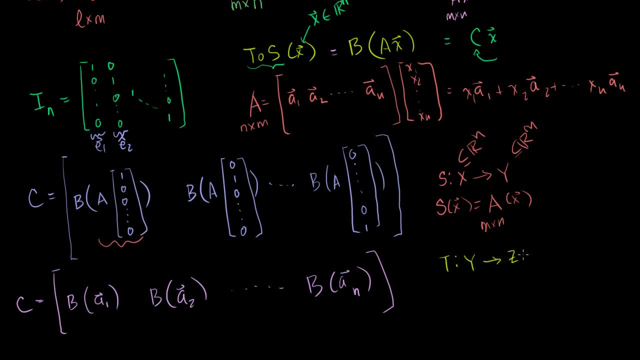 a mapping from Y to Z. Z is a subset of Rl And of course, T. the transformation T applied to some vector in X- sorry, in Y- can be represented as some matrix B times X. OK, OK. So this is a mapping from Y to Z, times that vector. 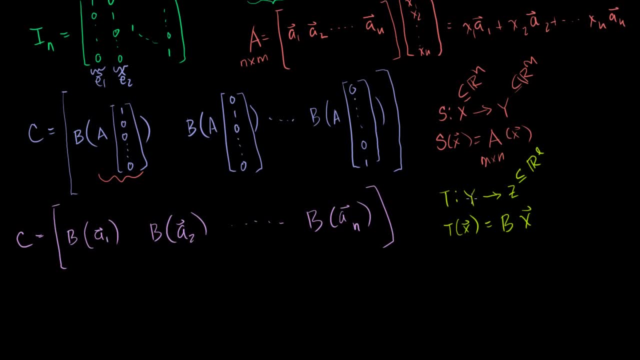 I shouldn't have drawn parentheses there, but you get the idea. And this, since it's a mapping from a subset of Rm to Rl, this will be an L by M matrix. And then we said, look, if we actually just take the 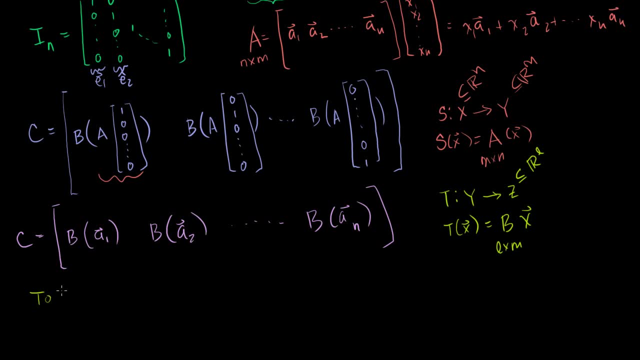 definition of. if we take the composition of T with S, this reduced to of some vector in X, this reduced to B. So first we applied the S-transformation, So we multiplied the matrix A times x, and then we applied the T-transformation to this. 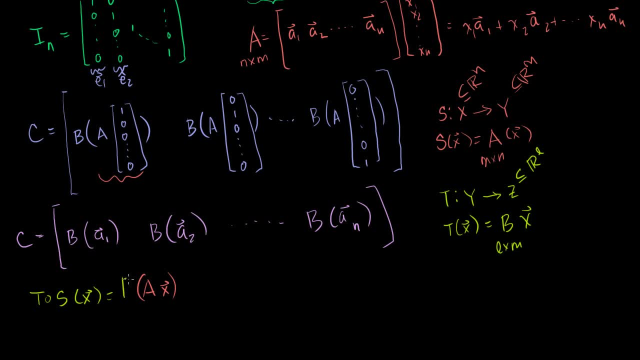 So we just multiplied B times that. Now we know that this is a linear transformation, which means it can be represented as a matrix vector product, and we just figured out what the matrix vector product is. So this thing is going to be equal to. this is equivalent. 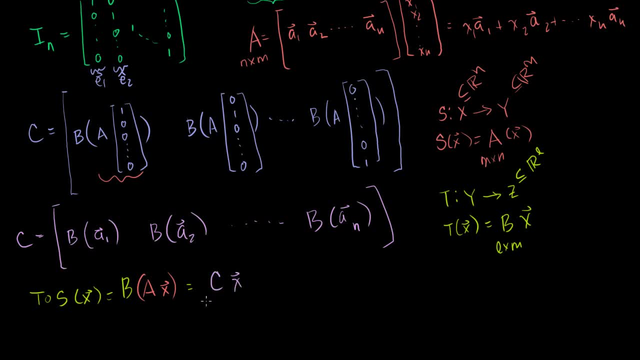 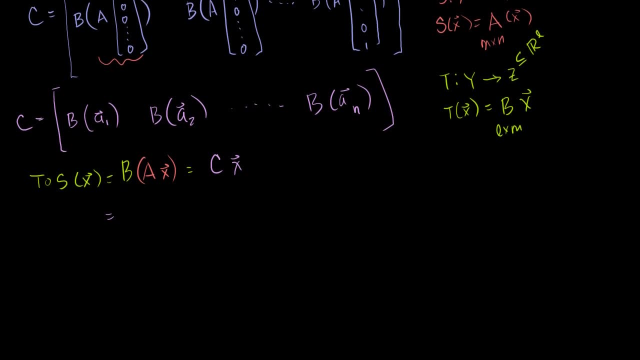 to switch colors, C times x, which is equal to this thing right there, which is equal to that thing right there, which is equal to- let me write it this way- B, B, A1, I'll try to be true to the colors- B, A1, where A1 is the first. 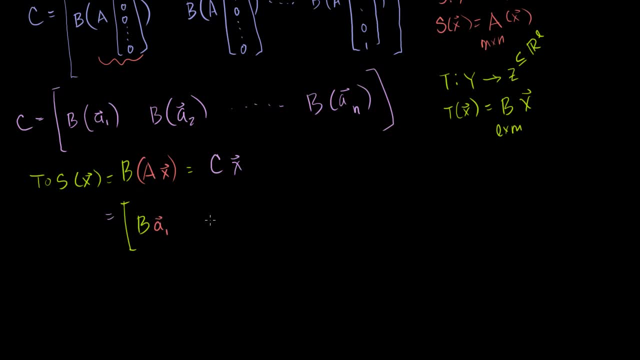 column vector in our matrix A, And then the second column vector in our matrix A, and the second column here is going to be B, And then we have A2, where this is the second column vector in A, and then you could keep going all the way. 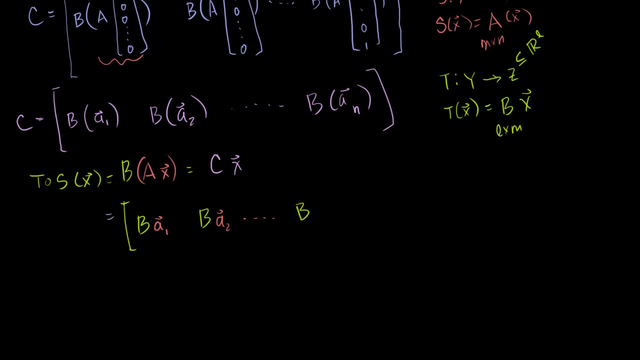 until you have B times An right there. times x, of course. times x. Let me maybe make it purple, Times x, Like that. Now, this is fair enough. We can always do this If you give me some matrix. remember this is an L by M. 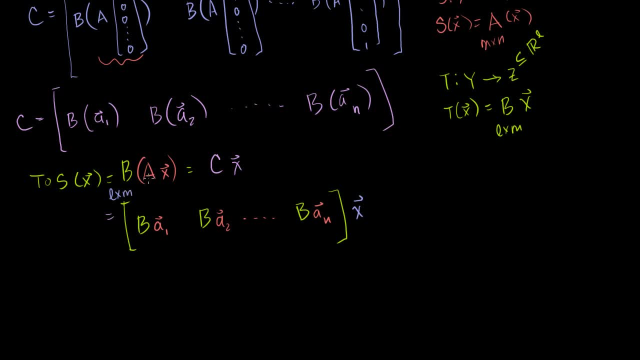 matrix and you give me another matrix right here. that is a M by N matrix. I can always do this, And how do I know I can always do that? Because how many entries are each of these? A's are going to have M entries, right. 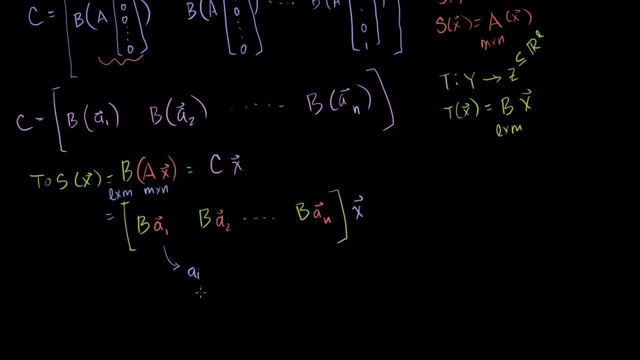 They're going to be. let's see A1, I say Ai. all of them are going to be members of Rm. So this is well-defined. This has M columns, This has M entries. So each of these matrix vector products are well-defined. 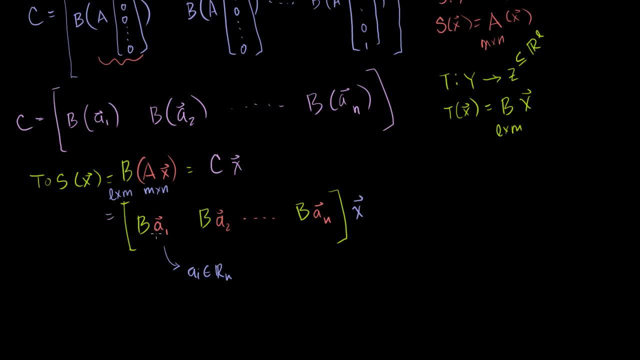 Now this is an interesting thing because I mean, we were able to figure out the actual matrix representation of this composition transformation. But let's extend it a little bit further. Wouldn't it be nice if this were the same thing as the matrices B times N? 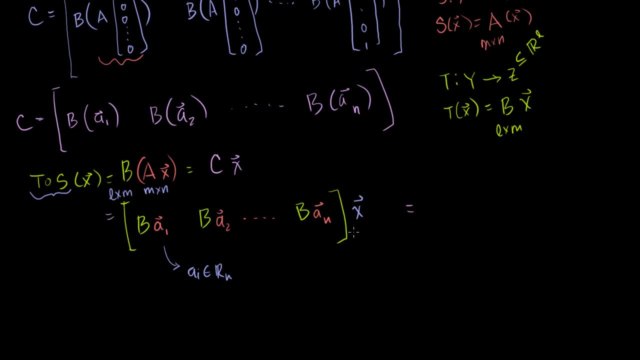 B times A. Wouldn't this be nice if this were the same things as the matrix B times. I don't want to write dot product, let me just write B times A. all of that times x. All of that times x. Wouldn't it be nice if these were the same thing? 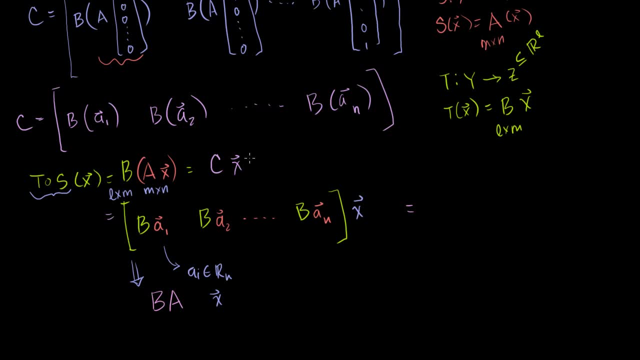 Because then we could say that the composition of T with S of x is equal to the matrix representation of B times the matrix representation of S, And you take the matrix representation of B and you take the matrix representation of S and you take the matrix. 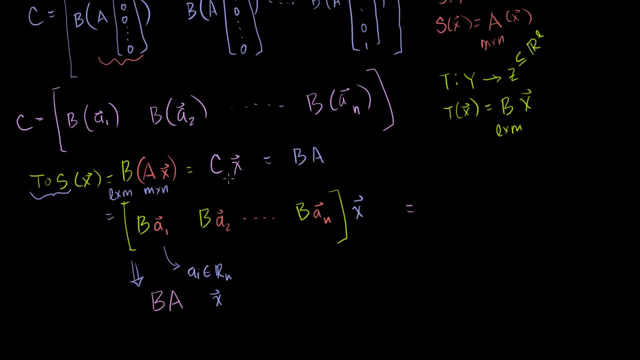 representation of B, and you take the product of those two and then that will create a new matrix representation that you can, which you could call C, that you can then multiply times x, So you won't have to do it individually every time, or do? 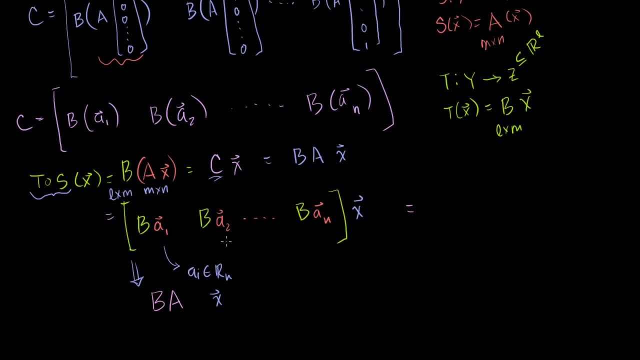 it this way, And I guess the truth of the matter is there is nothing to stop us from defining this to be equal to B times A. We have not defined what a matrix times a matrix is yet, So we might as well. this is good enough motivation for us. 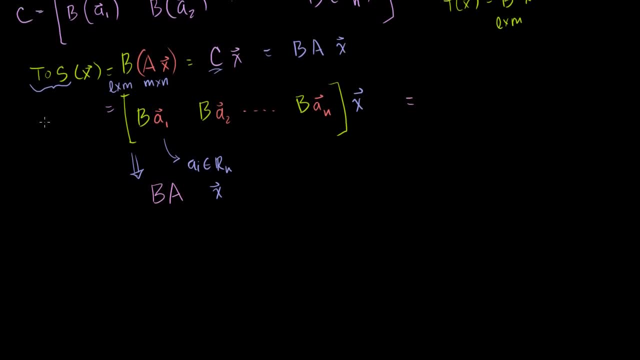 to define it in this way. So let's throw in this definition, Let us define. So, if we have some matrix B- and we could well- I don't have to draw what it looks like, but B is a L by M. 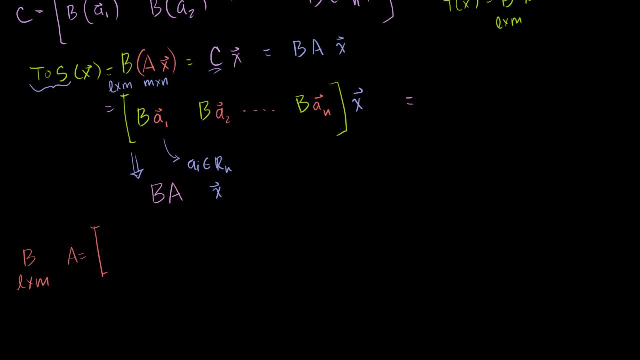 matrix. and then we have some other matrix, A, and I'll actually show what A looks like, where these are its column vectors: A1, A2, all the way to An. then we are going to define the product. So this is a definition. 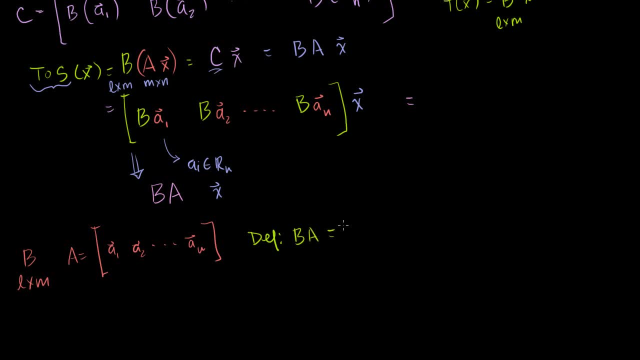 We're going to define the product BA as being equal to the matrix B times each of the column vectors of A. So it's B times A1.. That's going to be its first column. This is going to be B times A2, all the way to B times An. 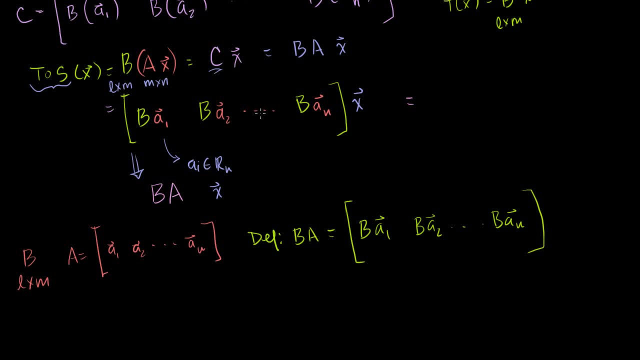 And you've seen this before in Algebra 2, but the reason why I did it- when I went through it I had kind of almost two videos to get to here- is to show you the motivation for why matrix products are defined this way, because it makes the notion of compositions of